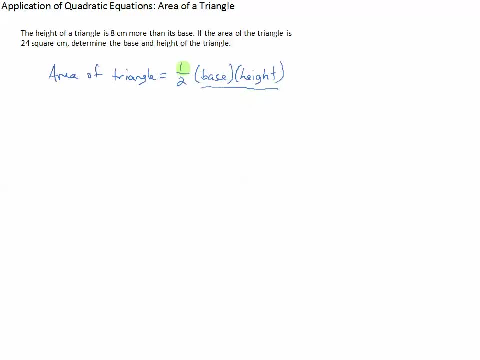 The area of a rectangle which is base times height, but it's half of a rectangle, so you have to multiply by half, Okay, so take account of that, And then the height of this particular triangle. if we were to draw a picture of this, let's draw some triangle here. It could be a right triangle. 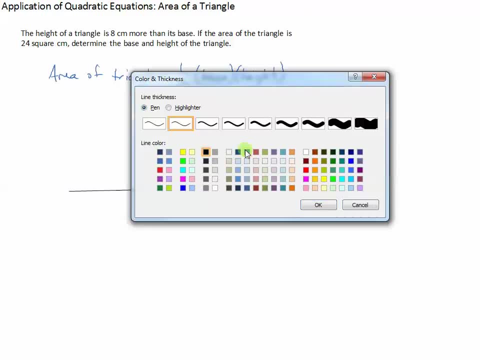 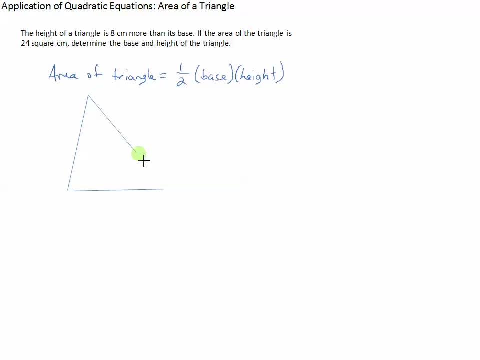 but I won't make that assumption. Let's change that color to match. So let's just say this triangle looks something like this And the base of it is, or the height is 8 centimeters more than the base. So what we'd do is maybe call the base something like x, since we don't know what it is. So x is the base. You could even write that off to the side: x is the base. And then, if x is the base, the height, which is like right here, the height would be 8 more than that, so it would be x. 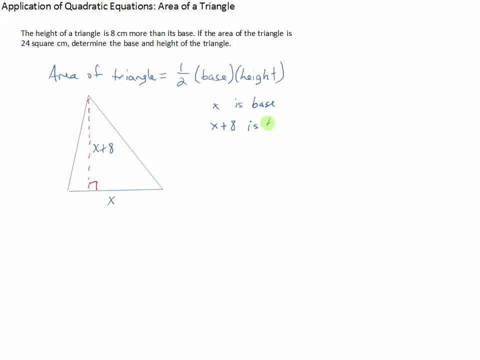 Plus 8.. So x plus 8 is the height. It's a good idea to write these things out, because now you can see that x plus 8 will be the height in this formula and x will be the base in the formula. 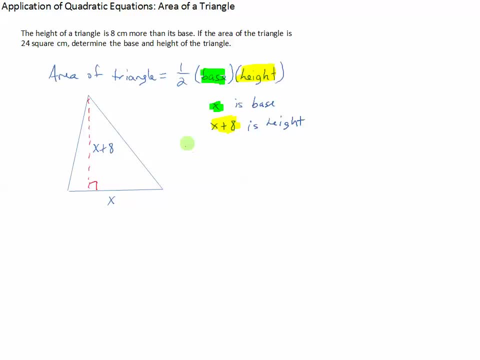 Okay, so what we end up with is we have to now create an equation. So what we know is the area of the triangle is 24 square centimeters, So that would be 24.. So we have 24.. the area equals 1 half times the base, which is times x times the height, which is x plus 8.. 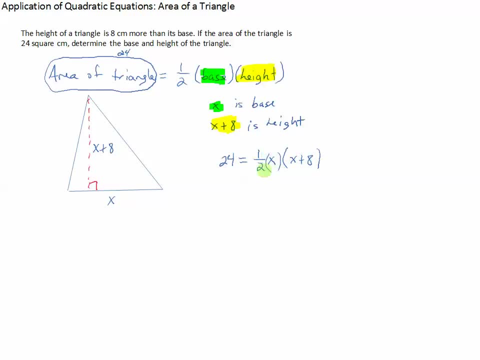 And in fact let's go ahead and put parentheses around the x. They're not necessary, but now we can see that there are three things multiplied. Now we just have to solve this equation. So I'll get you started, but I won't go into the details of how to solve it. 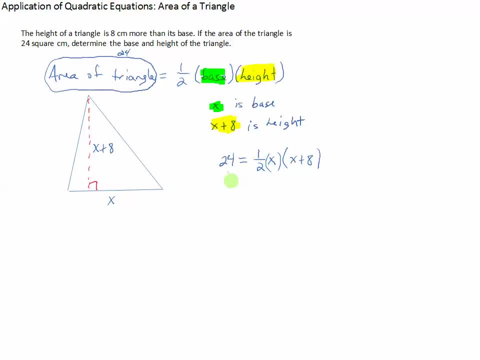 What I would do is multiply both sides by 2 first, To get rid of this 1 half. Now notice that the 2 does not distribute on the right side. These three things are not added or subtracted. So when you distribute, you only distribute over pluses and minuses. 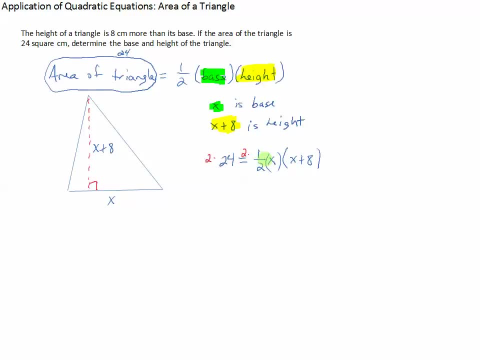 The right side is all multiplication right. It's 2 times 1 half, times x, times x plus 8.. So you simply multiply the 2 times 1 half And when you do that you get 1.. So on the left side we have 48..